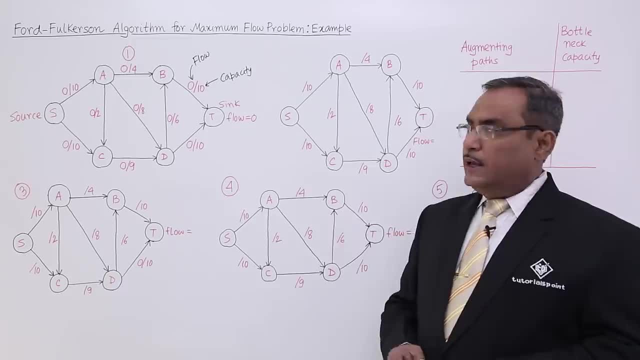 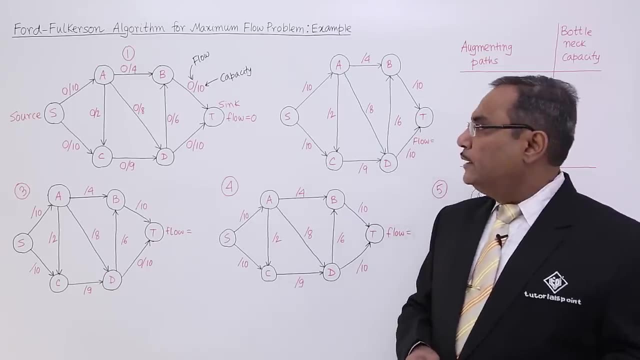 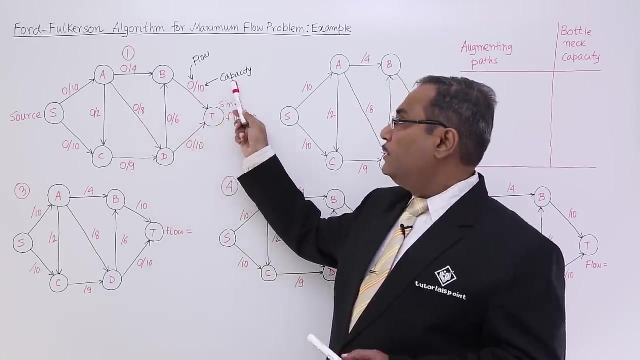 So here the source is S and sink is T And initially in the algorithm also we have mentioned that initially we shall consider flow is equal to 0. Now here we are having some integer value by some integer value. The second component will be denoting the capacity and the first component 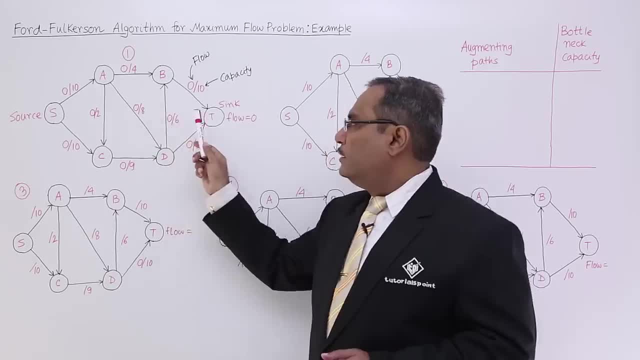 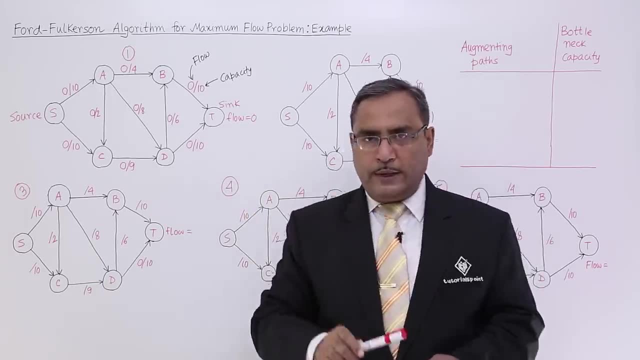 will be denoting the flow. That means from the source to the target, to the sink. the flow values are 0 initially, So that is why the net flow is 0.. So from here we are starting the algorithm. We know that in our algorithm we have mentioned three. 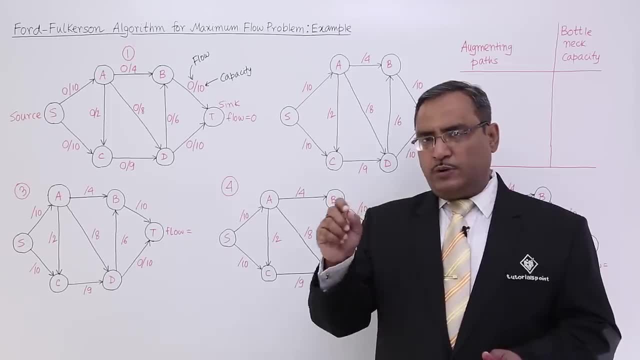 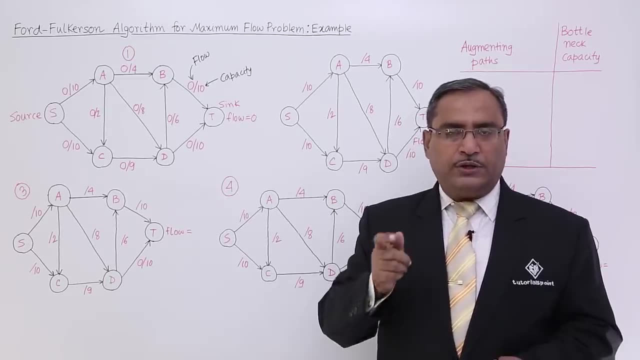 lines. we are having, statements we are having. First statement was: flow is equal to 0. And the second statement was: whenever we are finding some augmenting path from the source to the sink, then we shall go on computing the flow of that particular path and that flow will. 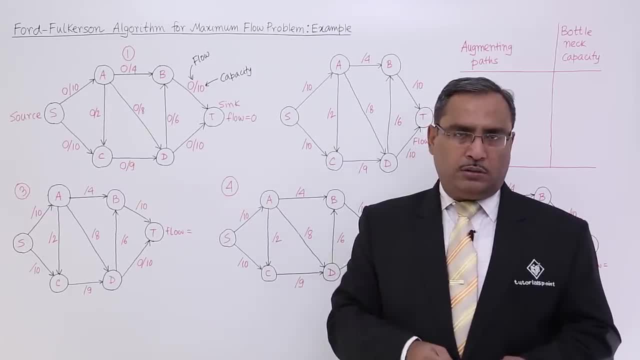 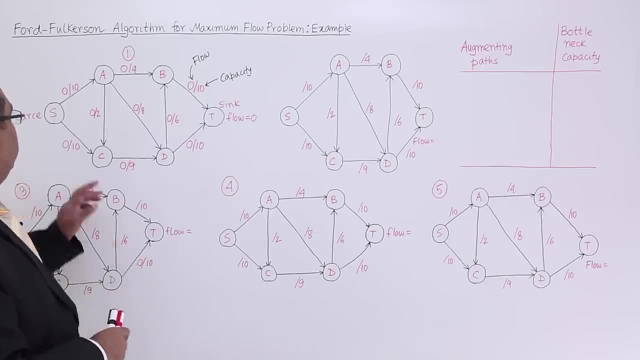 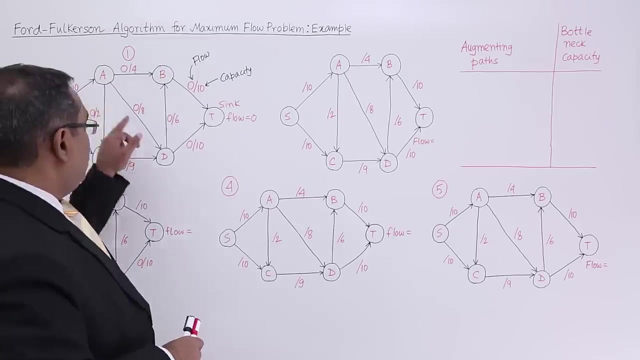 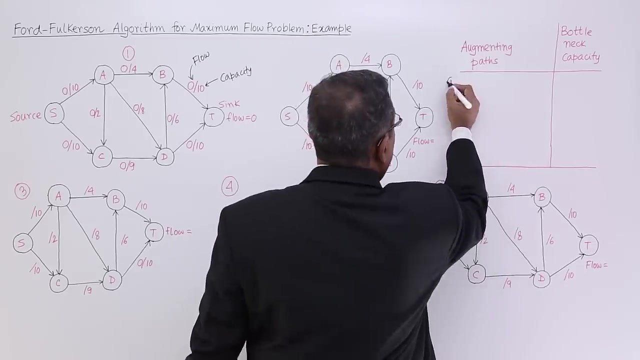 be added with the main flow. So now let me select one augmenting path. So at first we are selecting a path, say Sadt. Yes, the arrows are indicating that I can easily flow, So Sadt. So that is the first augmenting path we are taking, So I am writing the same here. path number 1: Sadt. 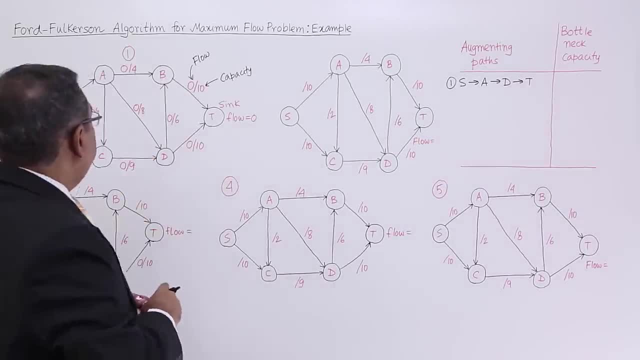 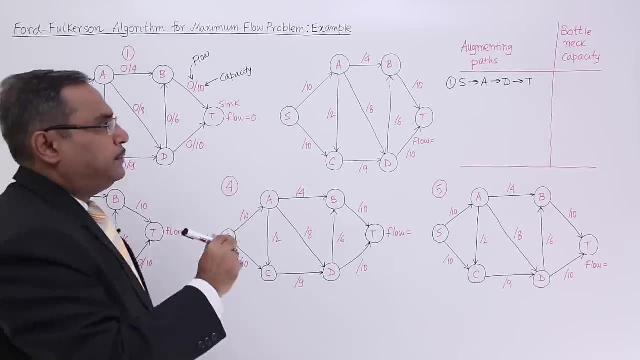 source to the sink. and here you see, here the capacity is that 10, 8, we are having 10 again, So 10,, 8 and 10.. So here the bottleneck capacity will be 8.. So the bottleneck capacity. 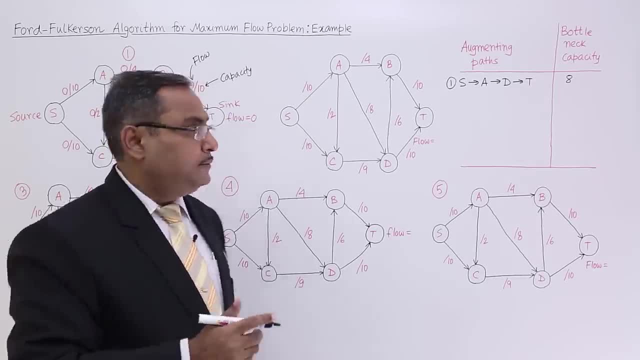 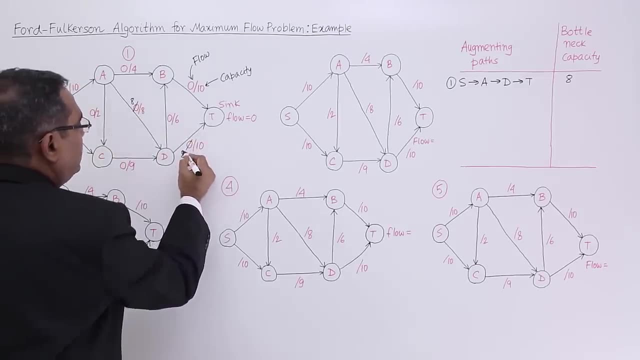 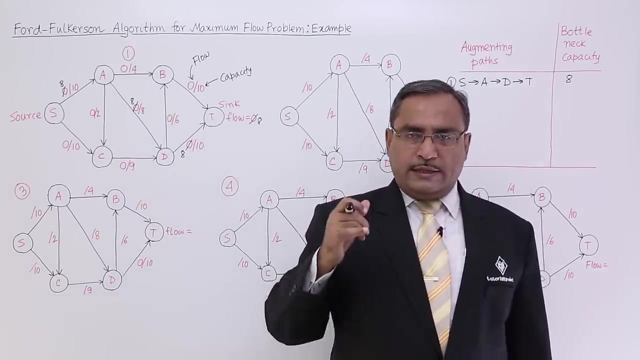 will be 8.. Now let me add this flow through this path, So it will become 8,, 8,, 8 and the flow will become 8.. So there is one augmenting path we have selected Now in. 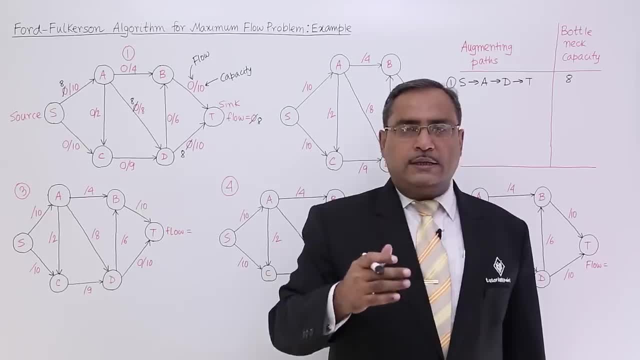 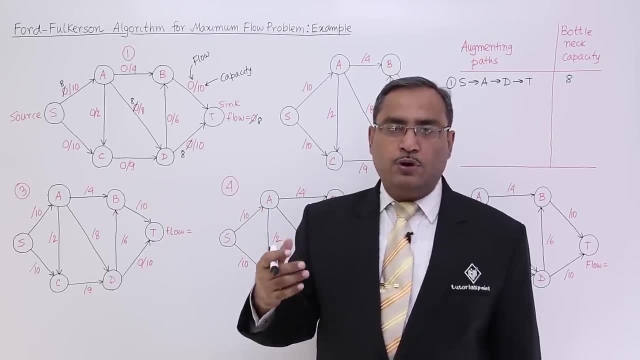 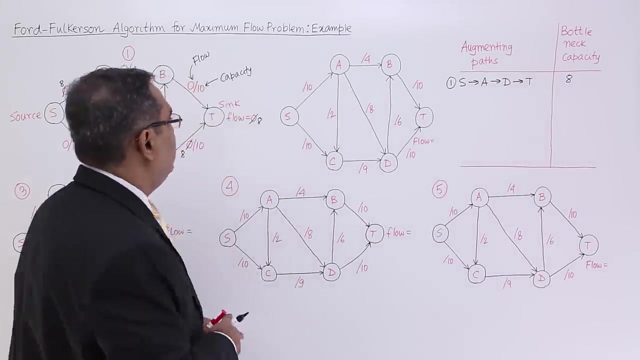 the second diagram. we shall write the updated values In the same diagram. I could have done the updates because that will not be easier for you to understand, So that is why I have drawn the same graph instance for multiple number of times. So now in the second. 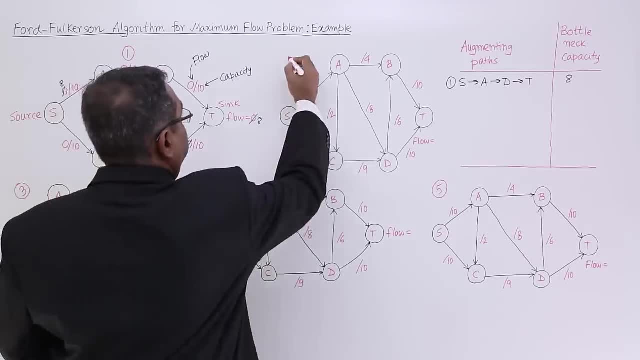 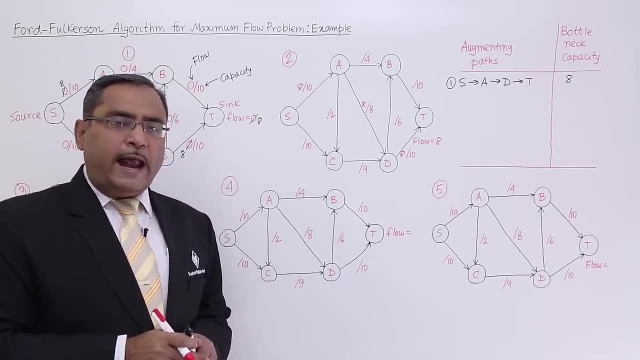 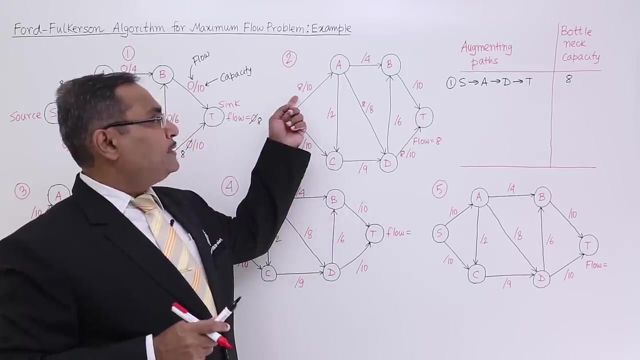 graph. there is a graph number 2, I am going for updates. So that is the graph number 2, updated version. Now we are considering another augmented path. but before going for selection of another augmented path here, you see it is having a capacity left as 2,. 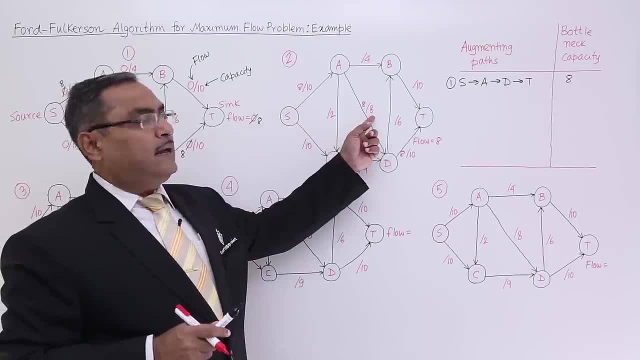 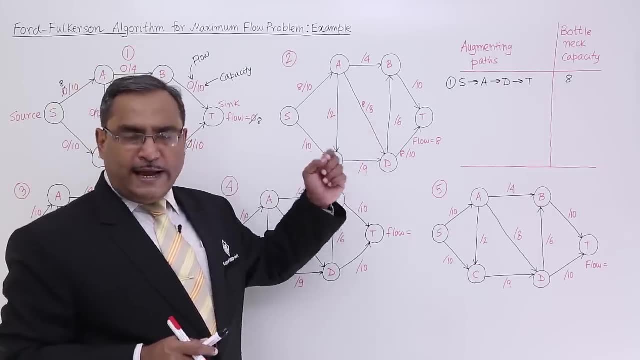 also known as the residual capacity It is having. the residual capacity is equal to 0 because flow is equal to 8 and capacity is equal to 8.. If you subtract flow from capacity, that is, 8 minus 8, you are getting 0, and here the residual capacity is 2 because capacity. 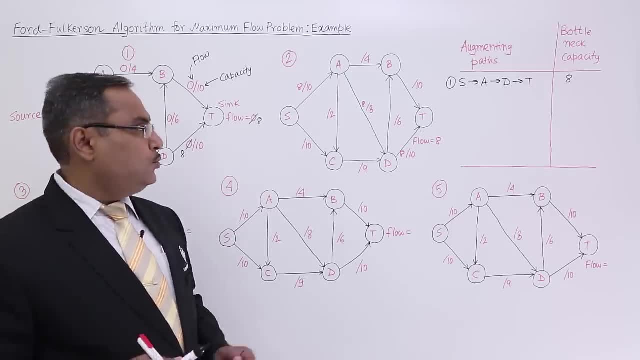 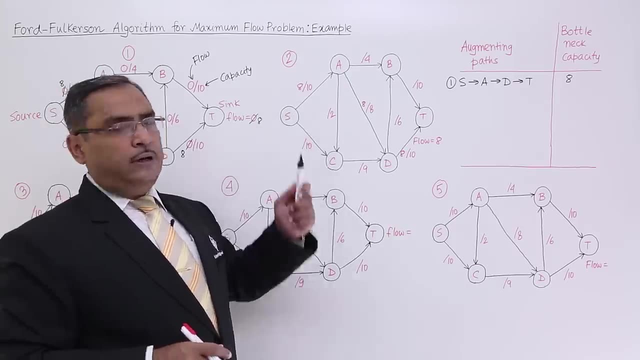 minus flow. if you go on subtracting 10 minus 8, you are getting 2.. So here the residual capacity is 2, here it is 0, and here the residual capacity is 2 again. So this particular path is capable to carry another. 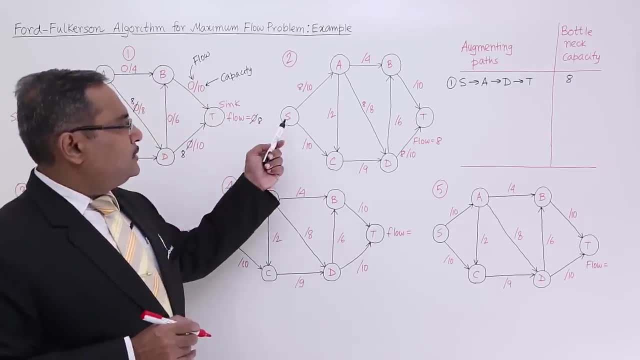 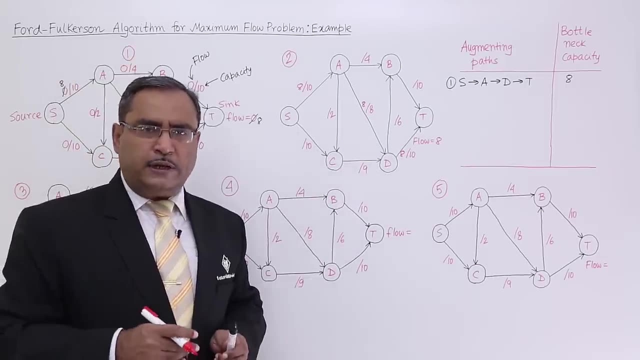 flow value of 2.. Now, the next path we are considering here, next augmenting path, is SCDT. Let us consider this one. I am selecting these paths very arbitrarily, So now, here you see. for the rest, we are having these 0s. 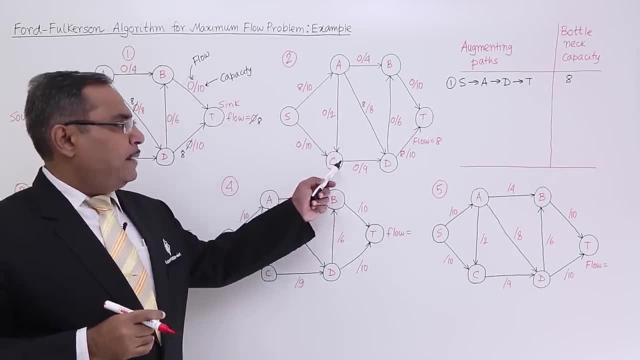 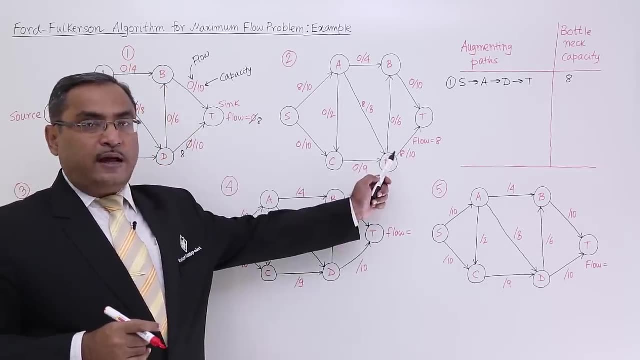 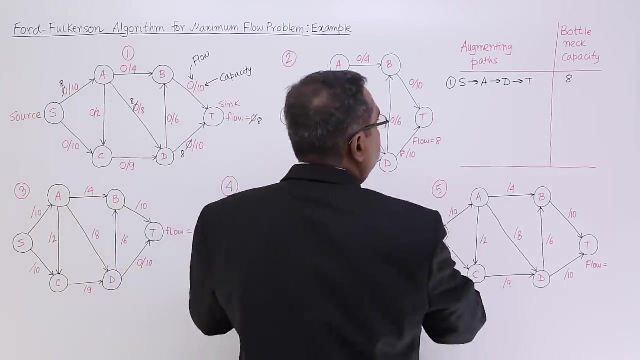 3.5.. see here the capacity is 10, capacity is 9 and the capacity here is 2.. So here the capacity is 2, because I should not consider the capacity, I should consider the residual capacity. So that is 2.. So now we are selecting the path like this one: Here the residual capacity. 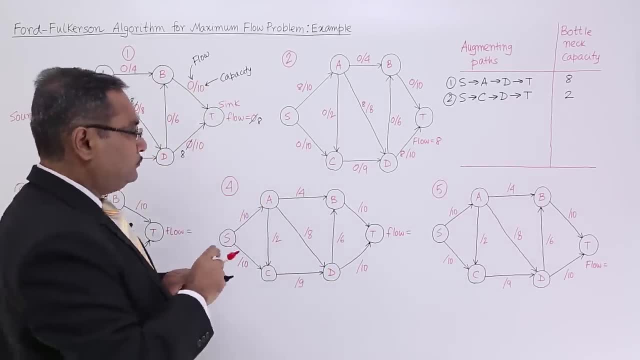 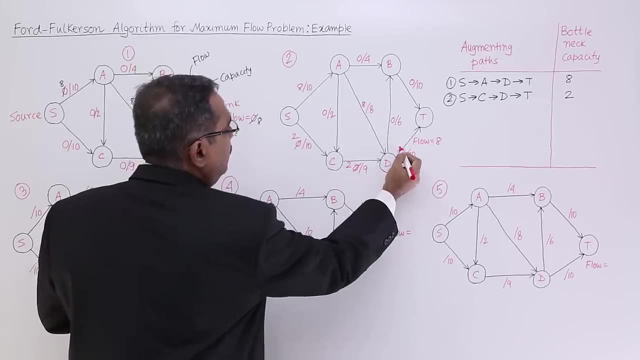 is equal to 2.. Now let me proceed. see here: I am giving this 2, this one is 2 and this one will become 10 and the flow will become 10. in that case, the flow will become 10 in. 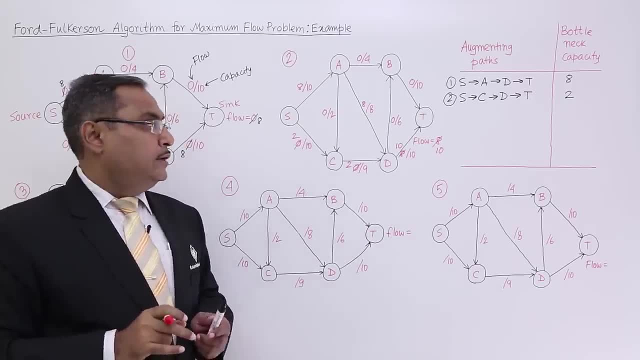 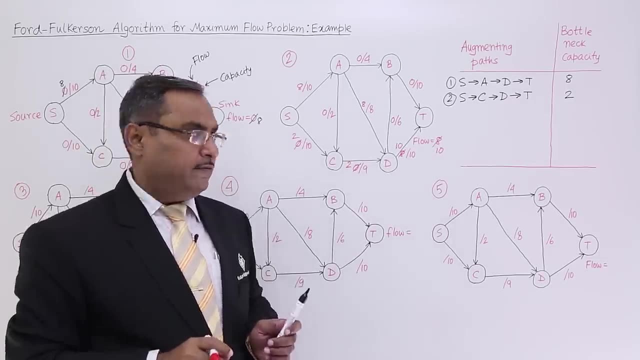 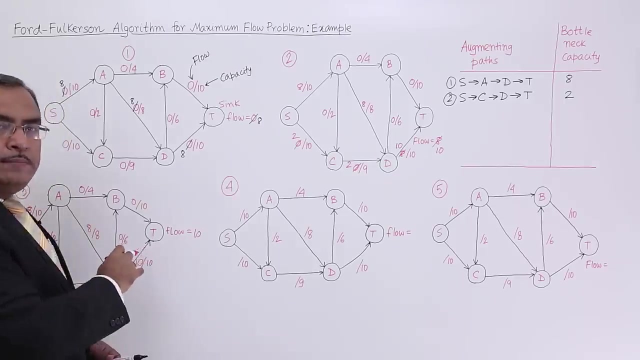 that case. So now it has been done in this way. ok, So the flow has become: 8 plus 2 is equal to 10.. So now let me do this. updates in the next instance of the graph. So I have completed my operations. So now just see what. whatever you have done from 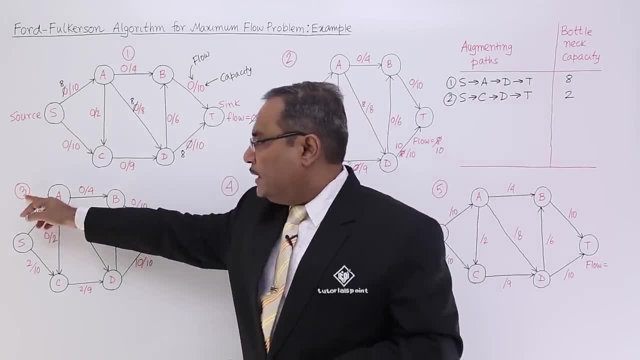 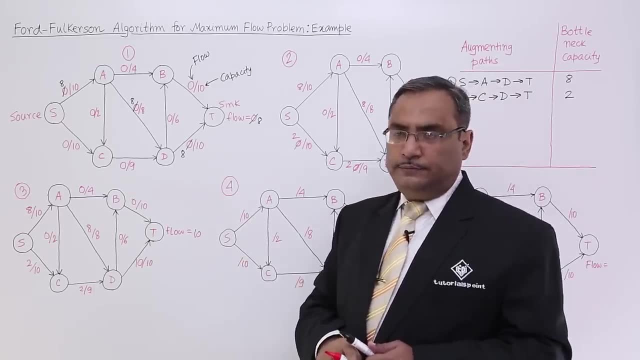 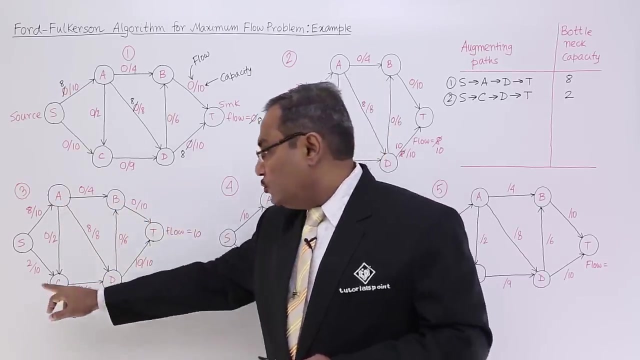 this very particular instance, number 2, this graph has got updated in the instance number 3 accordingly. I have just copied the values. Now, next path we are selecting, that is, your S C D A B T. So S C D A B T. 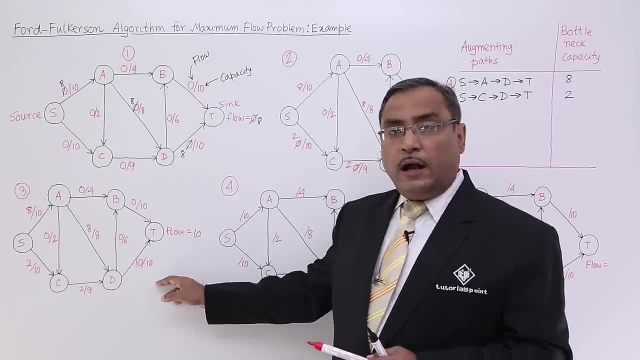 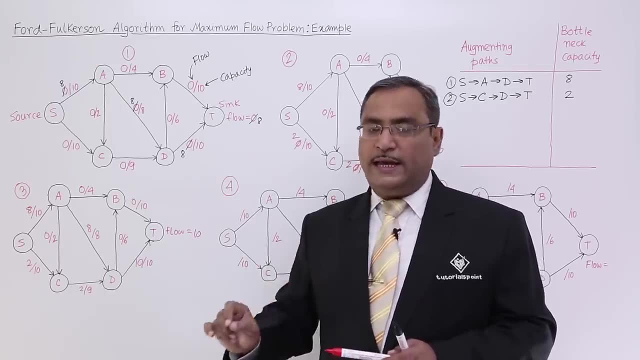 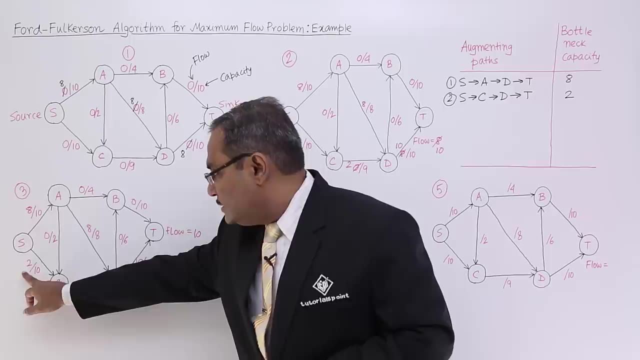 So now what we are doing. In our earlier videos we have discuss that we can select this augmenting path through those as S, which are non full forward edges, like this one. This is a non full forward edge. non full Why? because at the capacity is 2, flow is two. 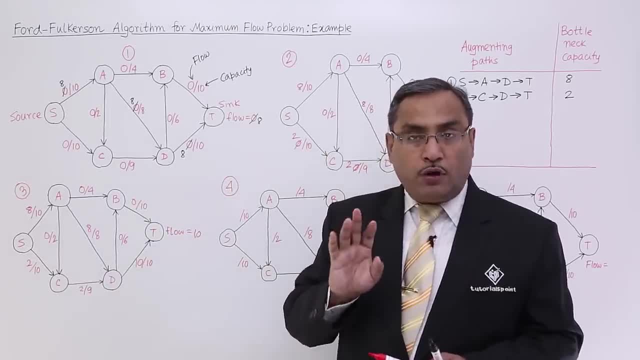 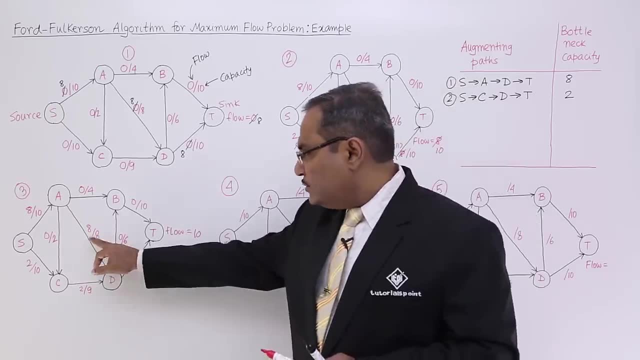 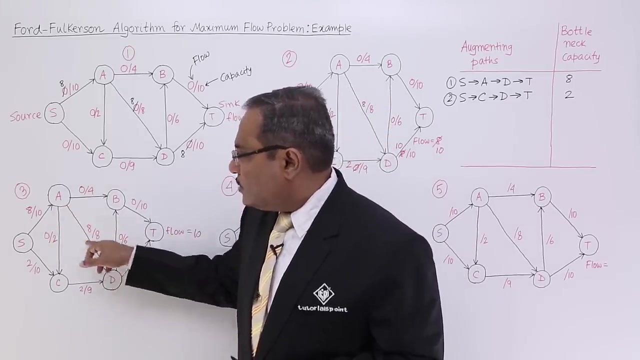 So the residual capacity is 8.. So that is why it is non full forward edge. And another and another one is non-zero backward age. So here you see the capacity. residual capacity is 0, but it is. if you consider this path in this way, there is a backward age and that 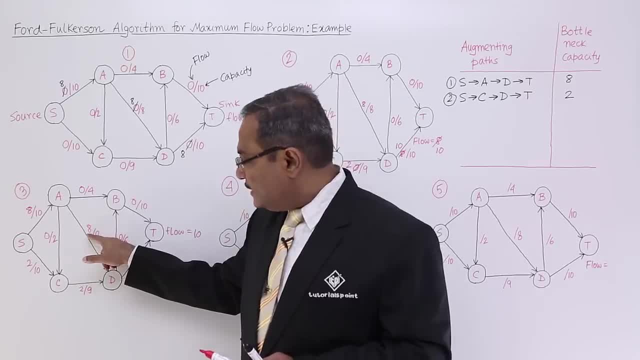 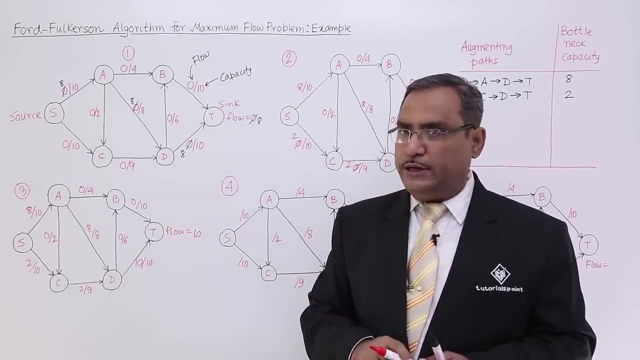 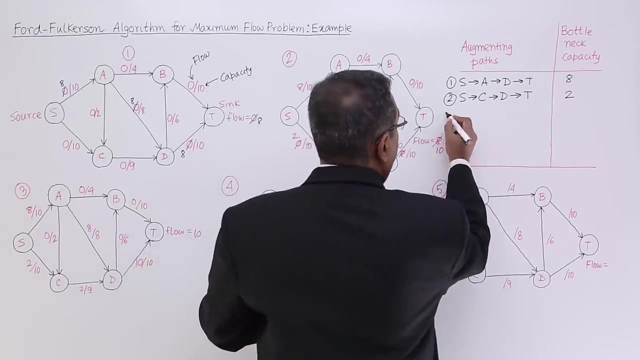 is the non, that is a non-zero. it is, yes, it is non-zero, it is 8.. So we shall select this particular path in this way. So now let me discuss this one into details. Now, what are the path we are selecting? I am just writing that one here: S C D A B T. S C D A B T. So 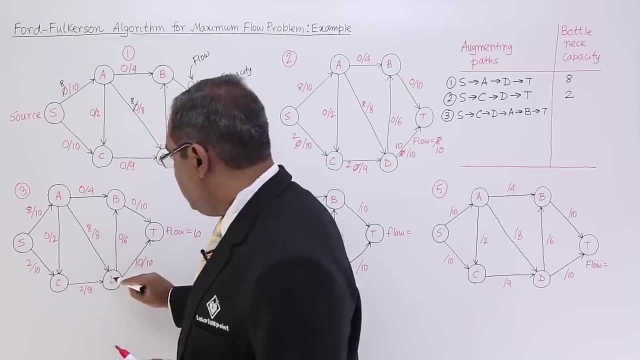 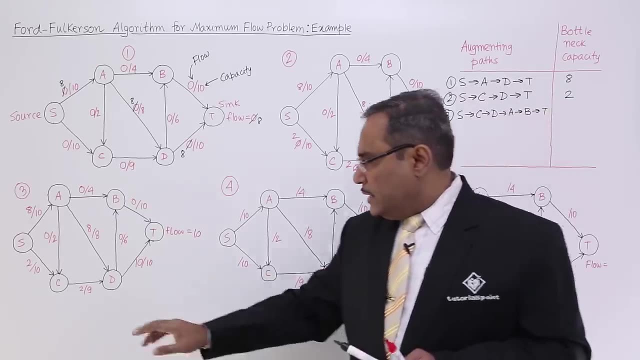 what is the path? So that is the S, C, D, A, B, T. So now let me find out the bottleneck factor. Here the value is 8, here the value is 7, here the value is 4 and here this value. 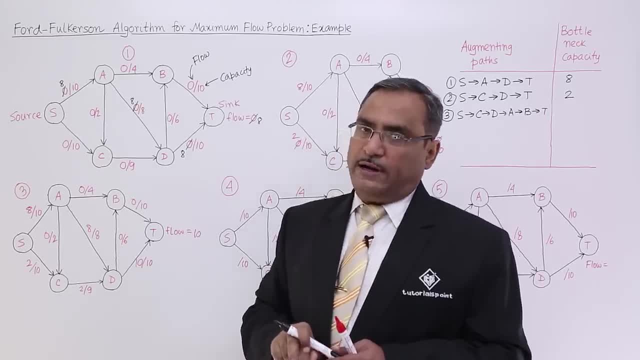 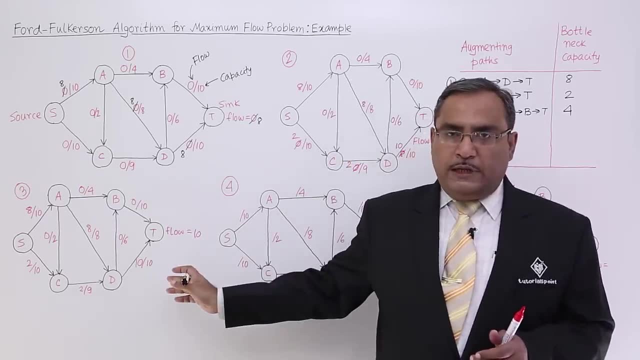 is 10 again. So I think 4 is 8.. So this is our bottleneck factor. So now we are going to this, So bottleneck capacity will be 4.. So now let me update this particular graph, see what happens. So I have done the 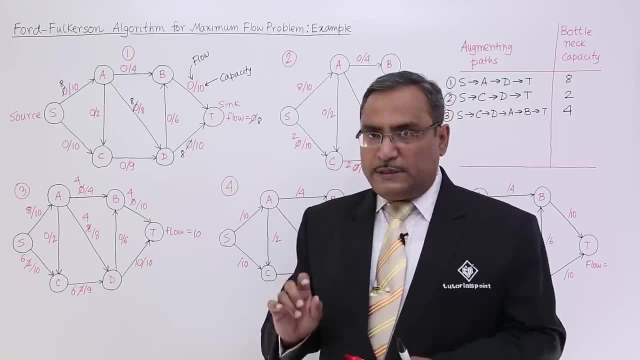 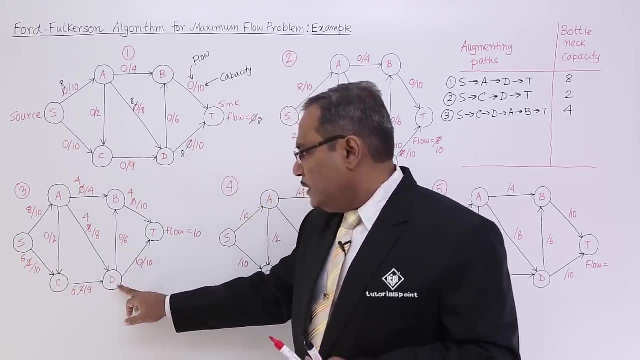 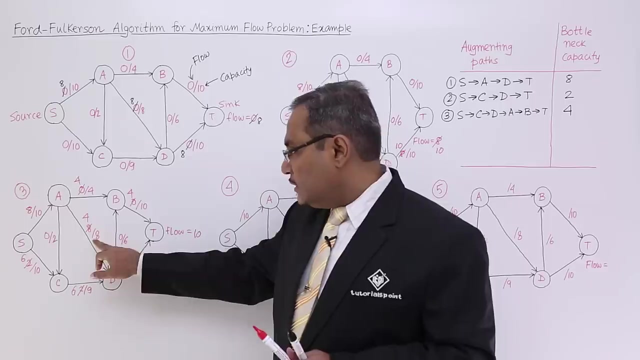 updations. see here the bottleneck capacity is 4.. So that is why 2 plus 4: 6 will be there. 2 plus 4: 6 will be there. and then there is a reverse path, So it is having having the non-zero flow here. So 8 minus 4, 4 is there, 0 plus 4,. 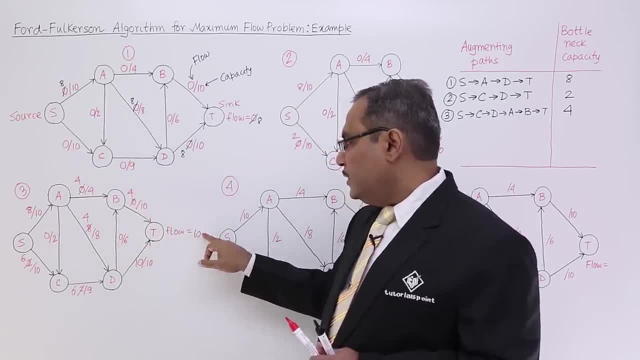 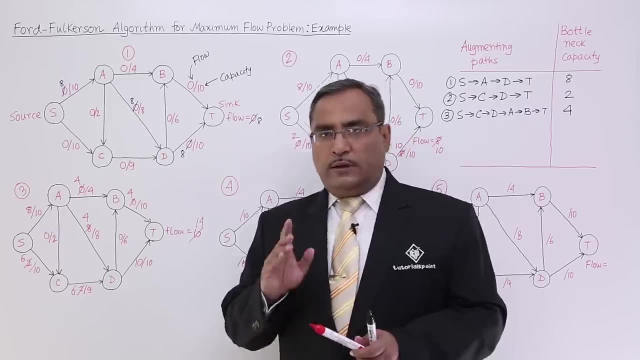 4 is there, and then 0 plus 4, 4 is there. in this way we are having- and here this particular flow with become 14.. Now see, in the earlier video we have mention that each and every vertex other than this source: 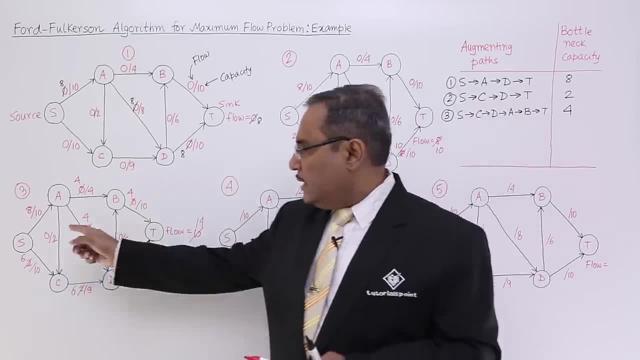 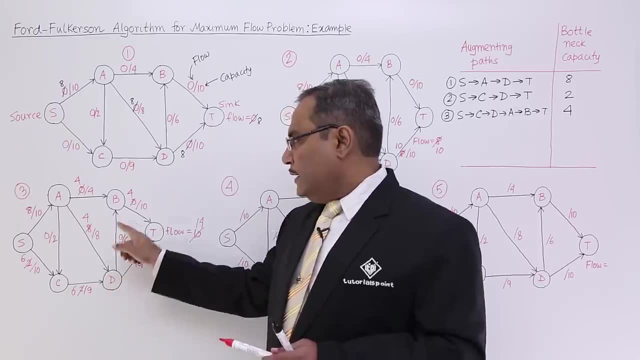 and sink should have the same inflow and outflow. Just see, here we are having this inflow to this node. a vertex a is eight. you see it has got distributed to four and four. here it is having the inflow of four, so it is having the outflow of four. here it is having the 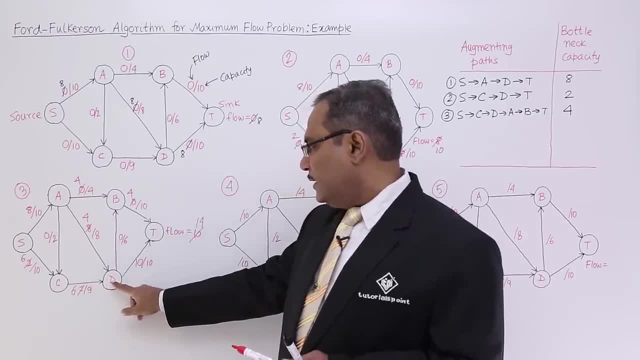 inflow of six. so that is why this inflow of six we are having and this particular inflow of six has been distributed- see, inflow of six has got distributed in this way: ten. why ten? because four is coming from this particular path, so this particular node is having inflow. 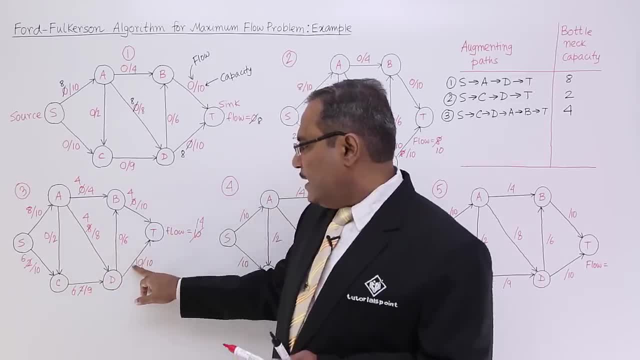 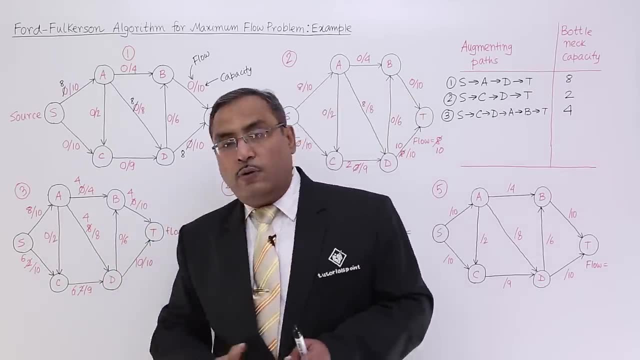 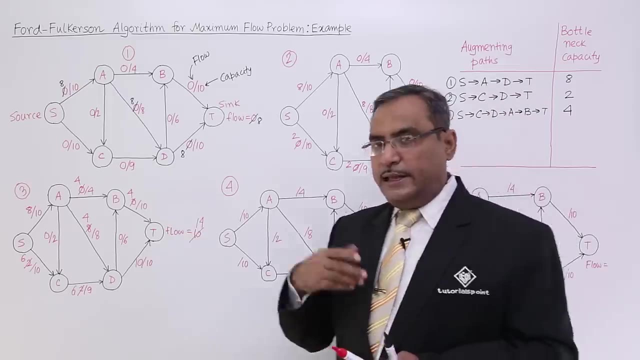 of four plus six plus four, that is ten, and ten is going to t. so each and every node other than this s and t, they are having the same inflow and outflow, so that has to be maintained. so for the instance number three to the instance number four, let me do the updates here then. 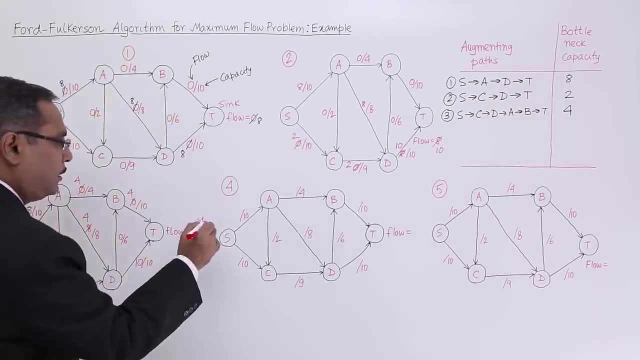 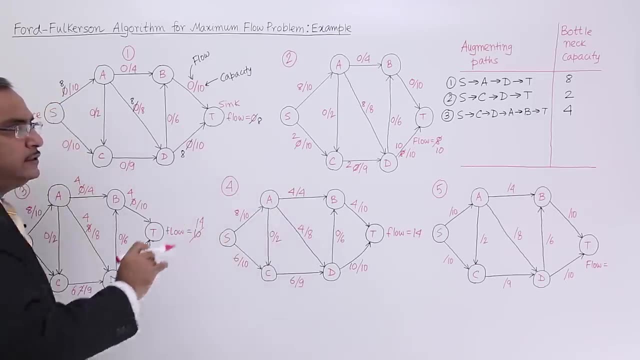 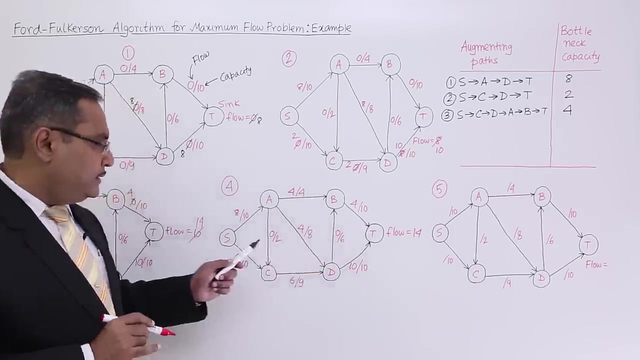 you shall select another augmented path. so i have done the updates. so now this is the final graph after the augmenting path number three. Now let us consider another augmenting path. now, here we will be considering the path like s, a, d, b, t. i am considering this one. why see here? the residual capacity is two here this. 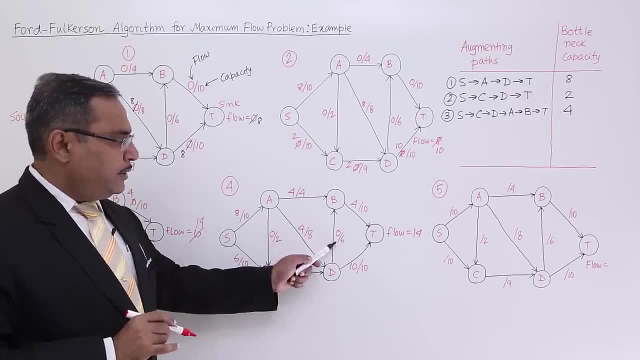 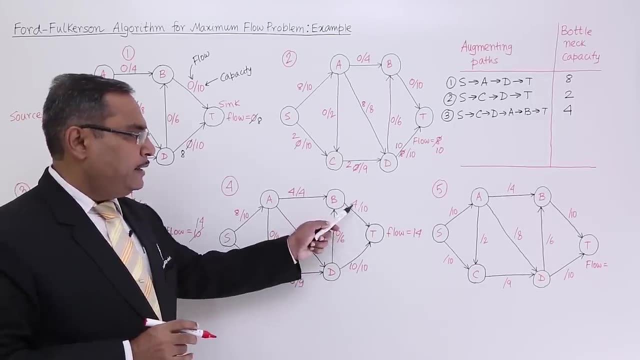 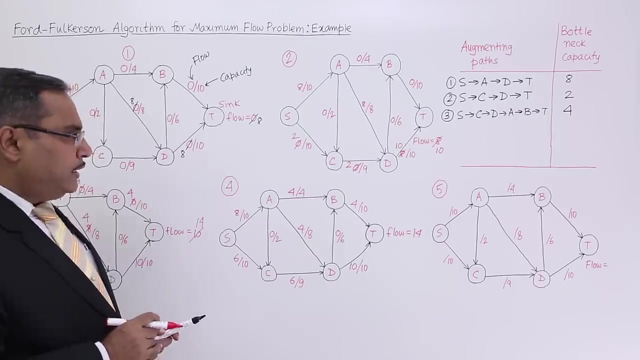 residual capacity we are having. it is four. here this residual capacity is six. so this particular edge we did not use earlier and here this residual capacity we are having is six again. so that is why i can proceed in this way. Now see what will be the bottleneck capacity. i think the bottleneck capacity will be two. 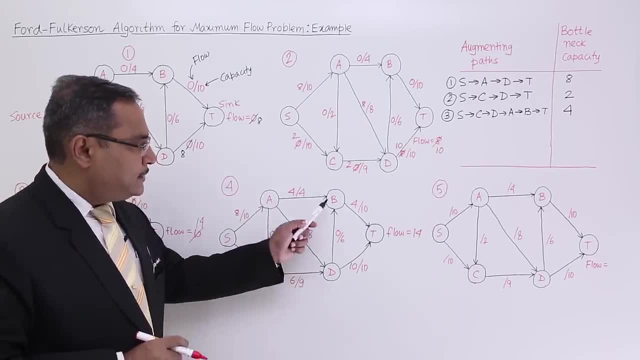 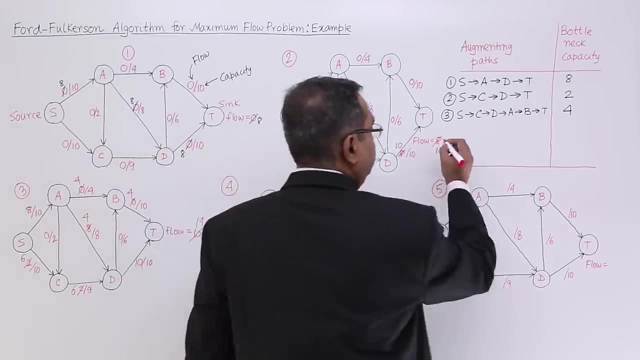 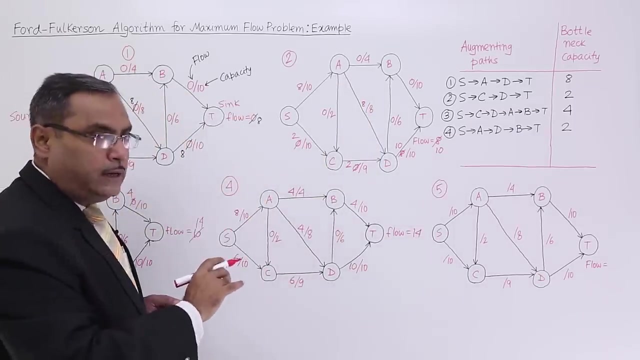 here, because it is two, it is four, it is six, it is six again. so here the bottleneck capacity will be two. so now let me write the augmenting path there. Now see, i have written the augmenting path. so now i am going for the implementation. so 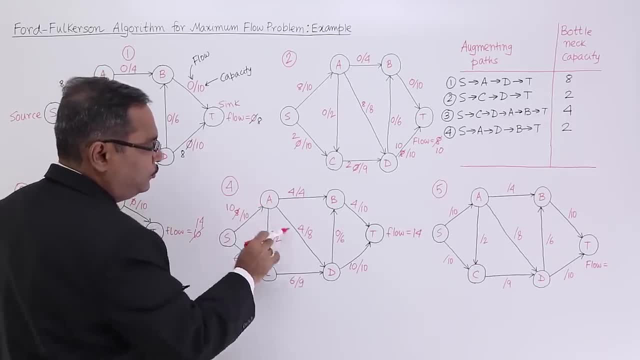 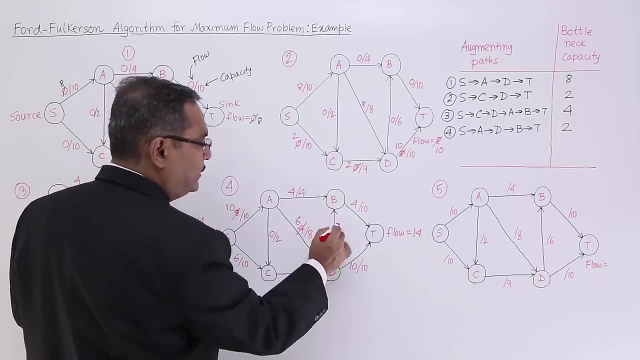 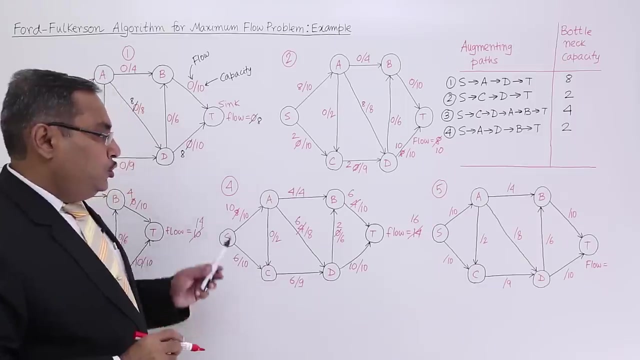 two will be added: s, a, then i should come to d, so two will be added. it is coming to d, and then it is going for d to b, so two will be added, and from b to t, so two will be added, and this particular flow will become sixteen. so in this way we have suggested the fourth. 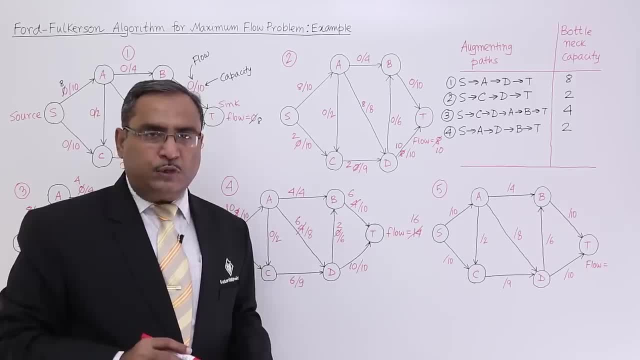 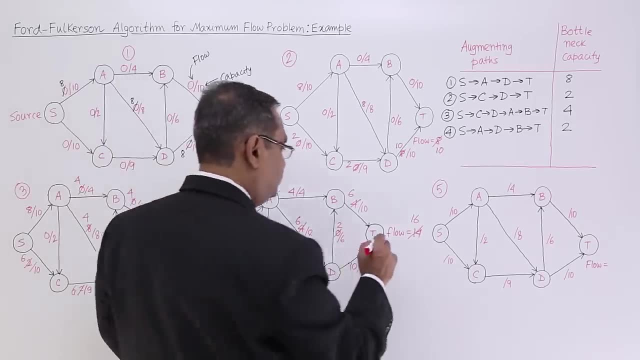 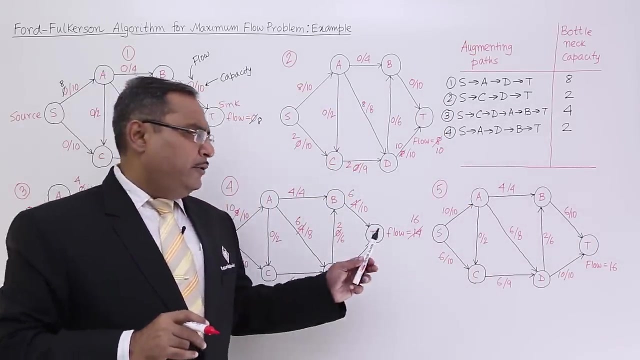 augmenting path. now let us try whether any other augmenting path is possible or not. so let me do the updates and that particular instance, number four of the diagram see. So in this way i have done the. i have completed this particular update. can you get any kind? 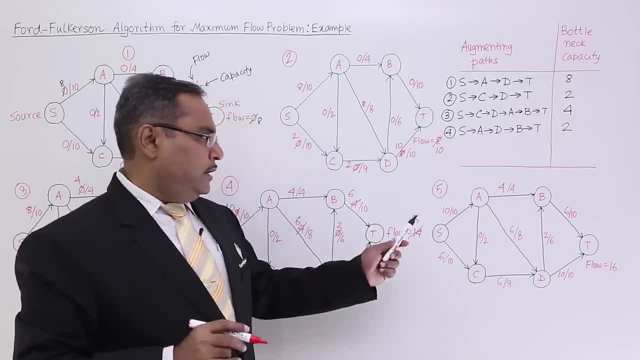 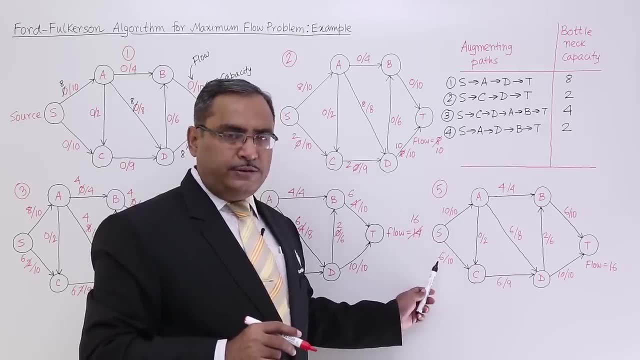 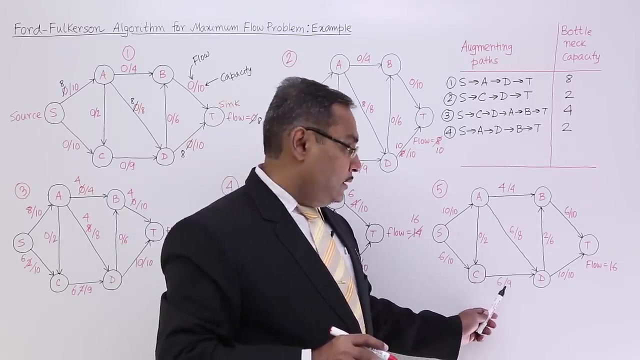 of extra. another augmenting path: here, you see, it is totally filled up. it is ten capacity and ten is the flow. here we are having some residual capacity of four, so it is coming down here. so now here we are having a residual capacity of three, and then we are having this: 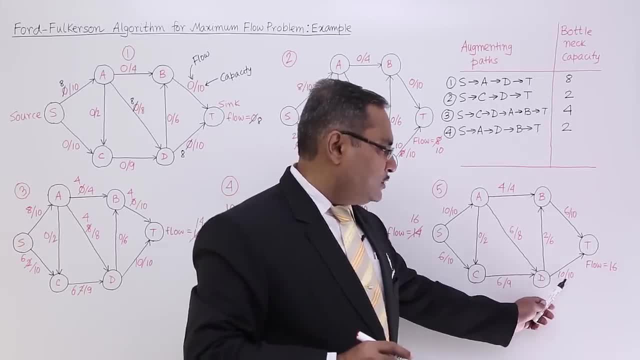 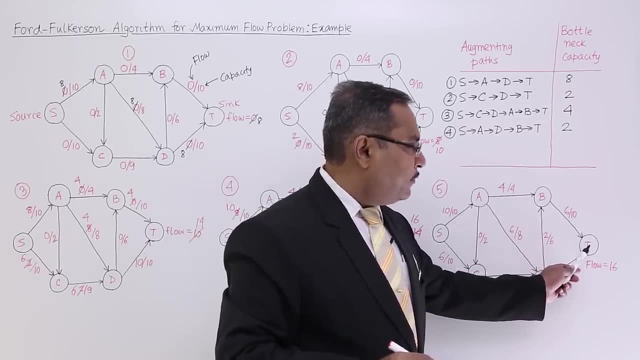 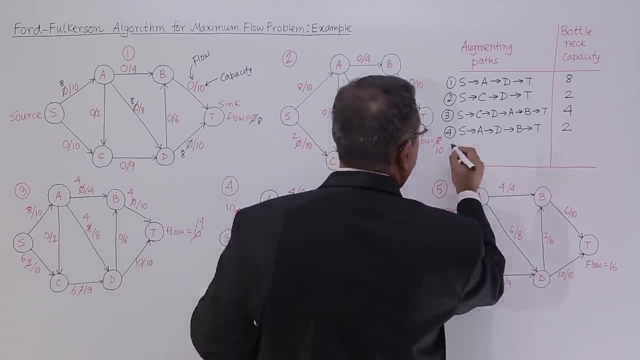 d. So now we are going for b. here the path is completely filled up, so i am going for b. so here the residual residual capacity is four and here this residual capacity is four again. so i can select another path like this. so let me write the path and here the capacity. 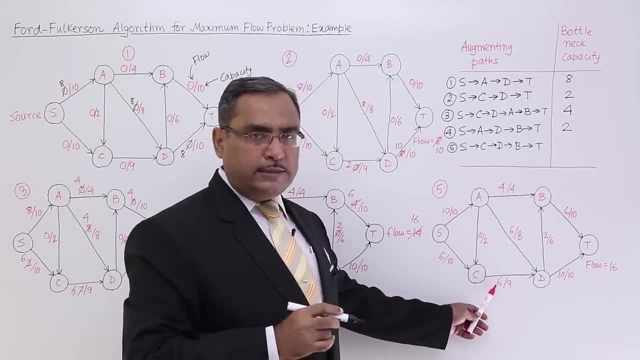 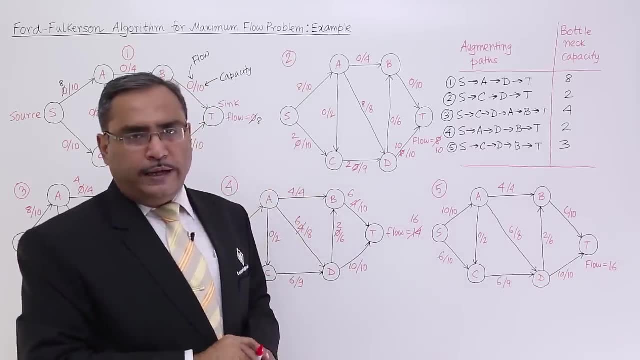 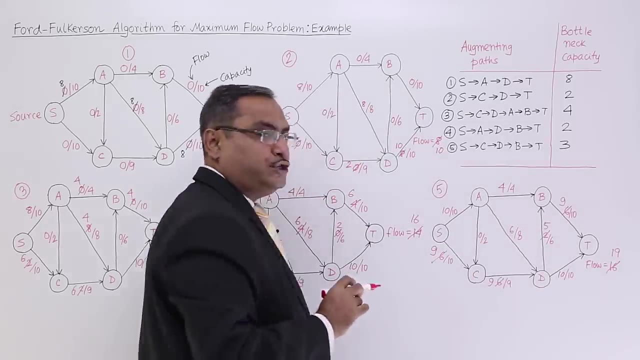 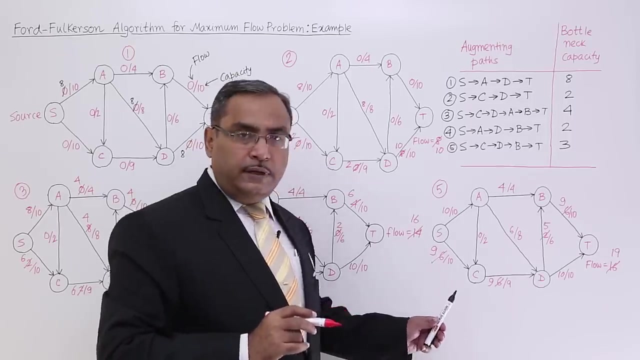 will be here four, and i think it is a minimum one. that is the three. so bottleneck capacity will be three. Now let me apply this one In this particular graph. see. so i have done the calculations accordingly now see. so in this way i have got the updates in this particular graph. can i suggest any other augmenting path? 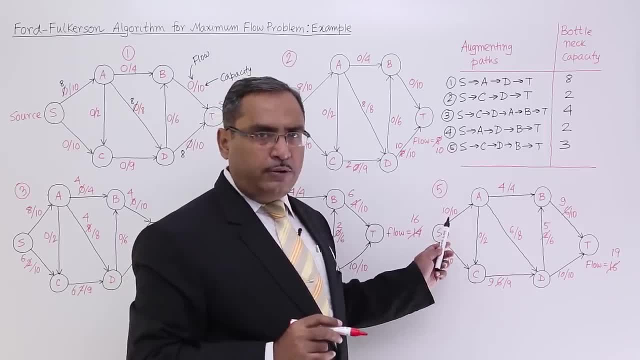 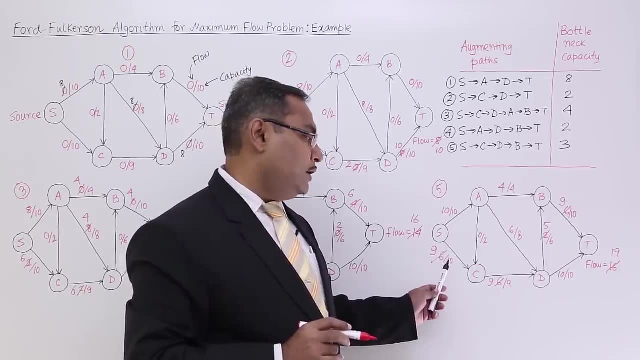 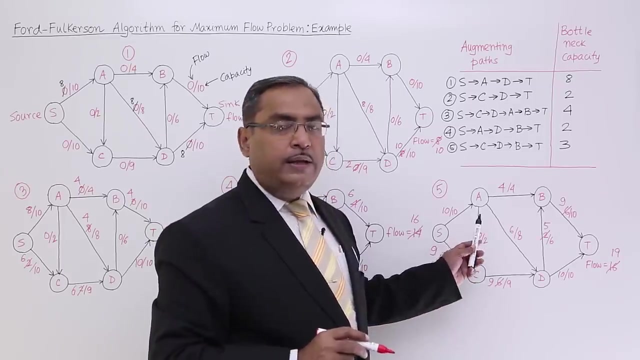 check here. path is not possible because it is having the value ten and ten. here one capacity is left, flow is nine and capacity here is one ten. so that means residual capacity is one. So here it is completely filled up. i cannot have this backward. why? because here this particular 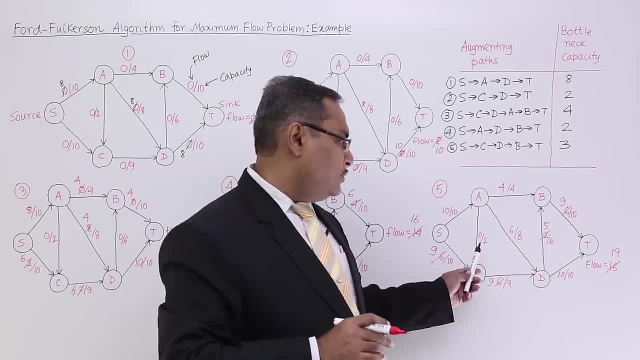 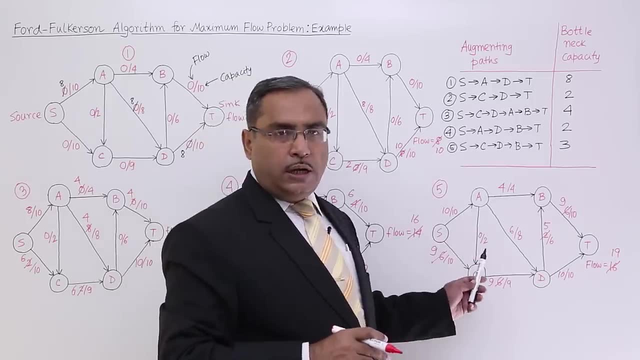 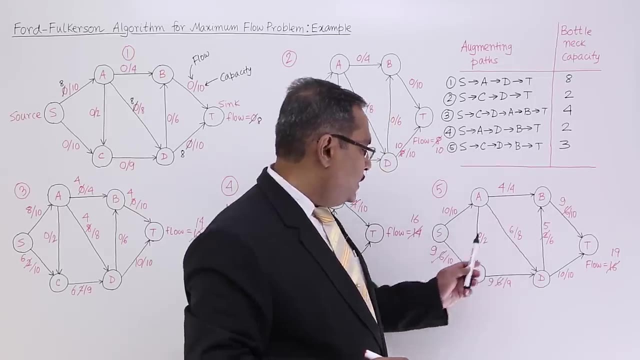 flow value is non zero is false, it is zero. so it flow value is not is not non zero, it is zero. So that is why the backward, backward movement is not possible. so now, so that is why it has been blocked. it has been blocked from here. it has been blocked, so i cannot suggest any. 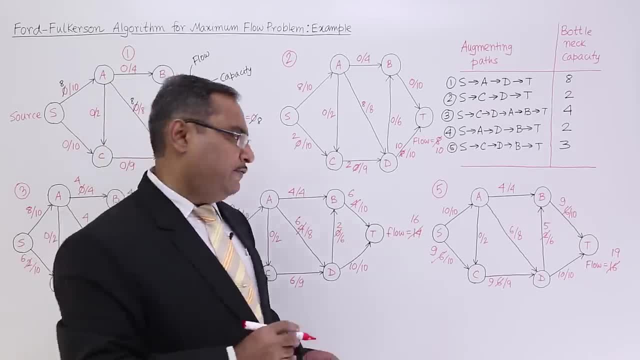 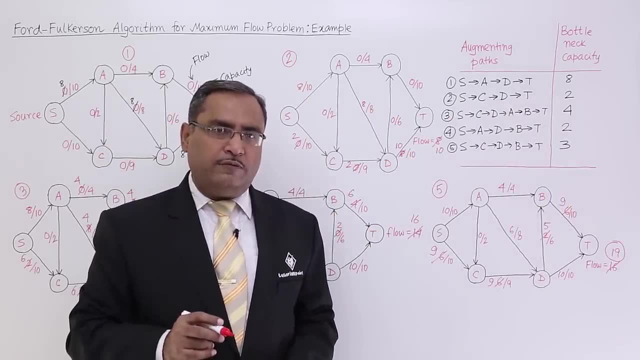 other augmenting path to this particular flow. Enjoy. Thank You, Thanks, graph. So now I think the answer will be 19.. So thus we have got this maximum flow for this network graph is 19. So in this way the values can get calculated, So all the instances are. 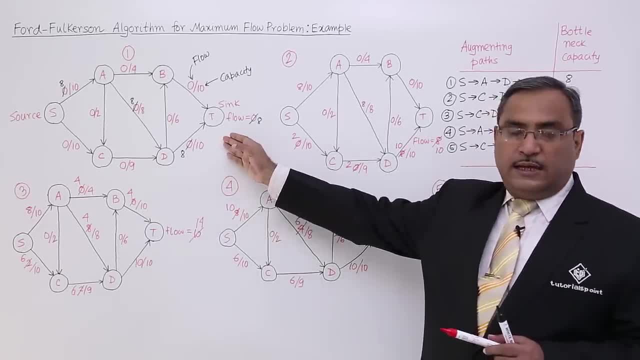 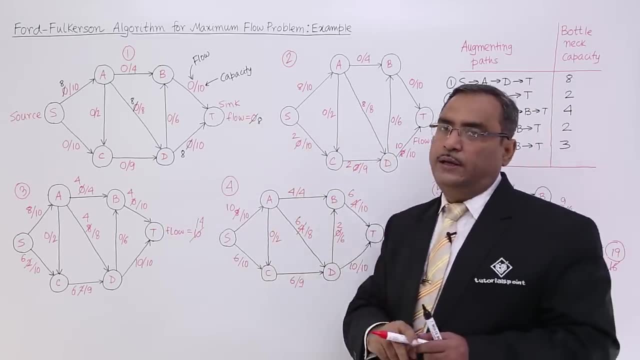 there in front of us. So there is a first suggested augmented path. after that then the second suggested, third, fourth and there is a fifth one. In this way we have solved this problem. So let me mark these paths for the better understanding to you. 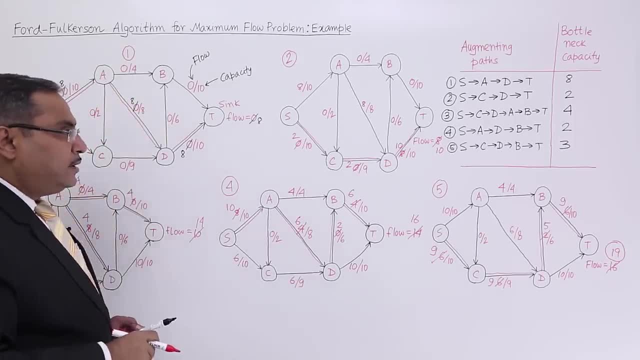 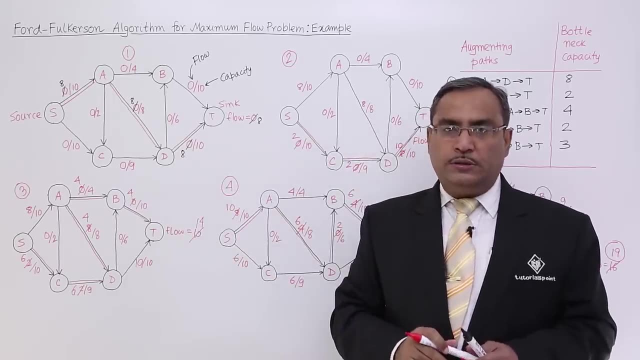 I have marked all the paths in the all instances of this particular graph so that you can get that which path has been selected in which instance. So this is the solution. In this way you can go for the solution Here. the solution value- maximum flow value- is 19 possible for this. 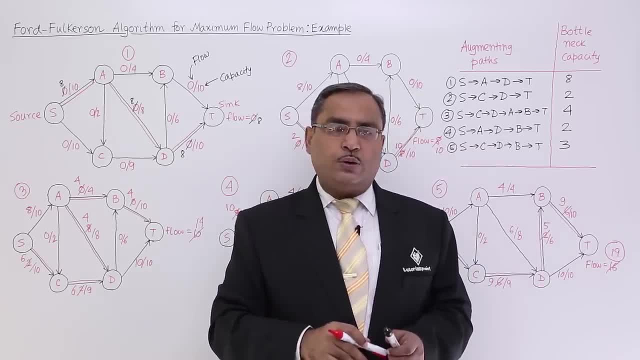 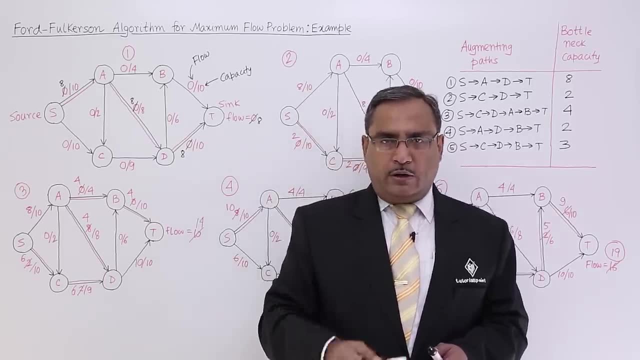 given network. So in the next video we shall see how to solve this problem. So let me mark these paths for the better understanding. show you how to calculate the complexity of this particular algorithm. So please watch the next video, because that video is in the continuation of this one. And thanks for watching this one. 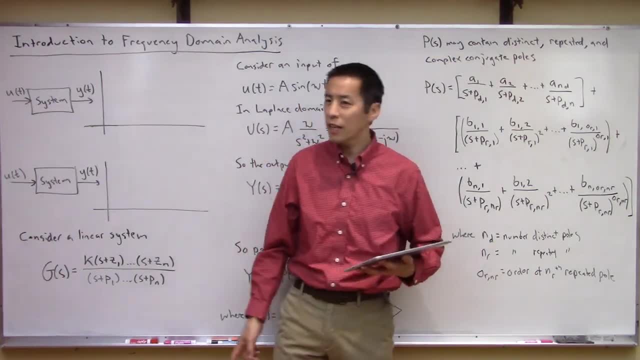 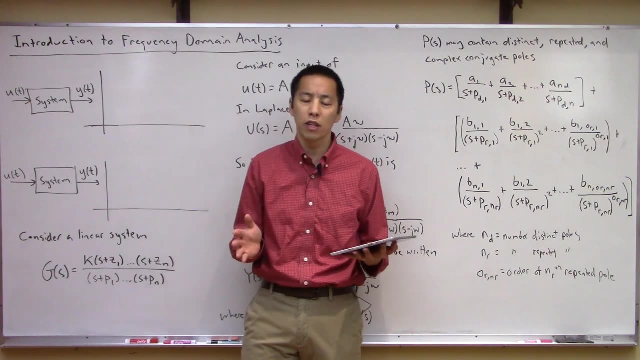 Hello everyone and welcome to another video. So today I'd like to talk a little bit about an introduction to frequency domain analysis. So, if you've been following along with the series, in the past we've talked a little bit about time domain analysis, which is really a fancy way of saying what does the system? 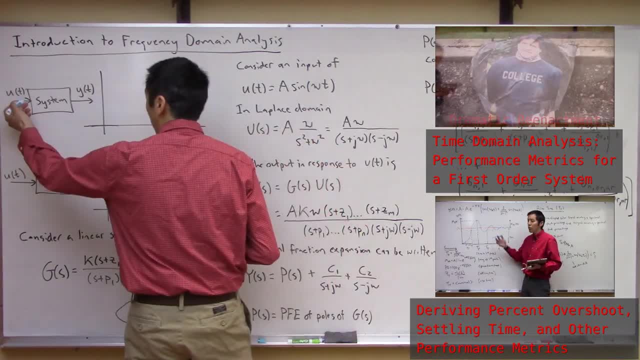 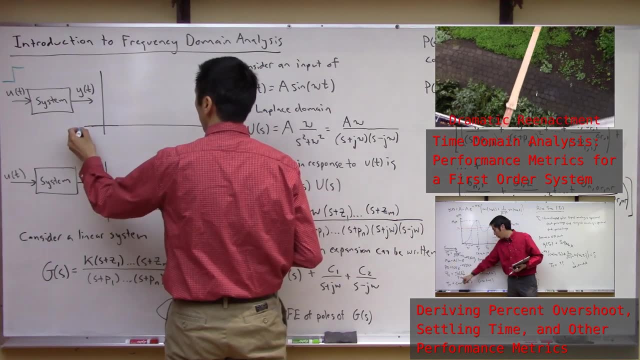 do if you have some kind of input to the system, For example like a step input. right, We looked at time domain analysis and we said, okay, what this system might do is, as soon as you hit it with a step, you know it does something like this, or